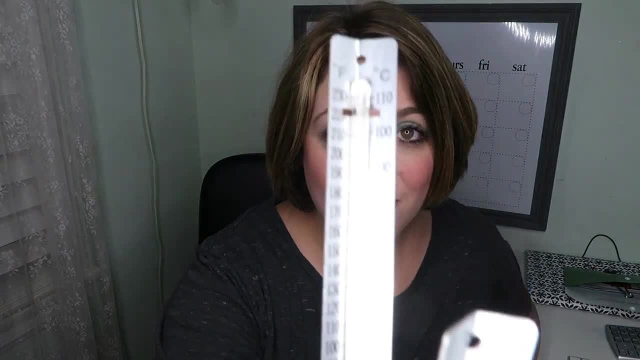 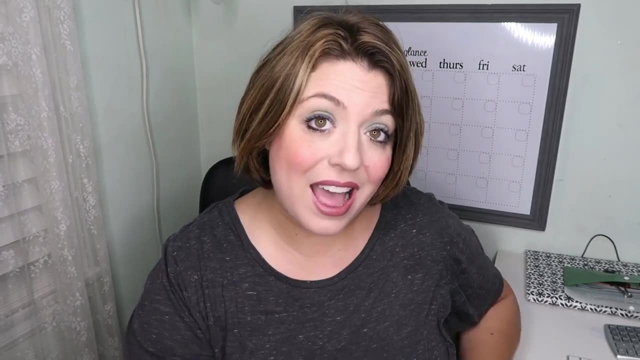 of glass. they're good quality and they have the degrees written on them very nicely. And just so you know, if you are in my community and one of the tutors with the Pasadena California community, I have purchased enough thermometers for all of you. So the day of community day on our Friday. 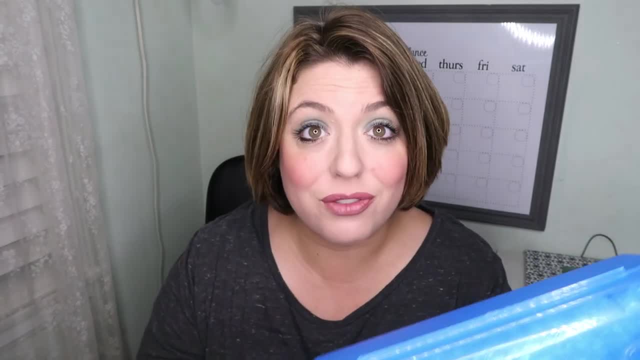 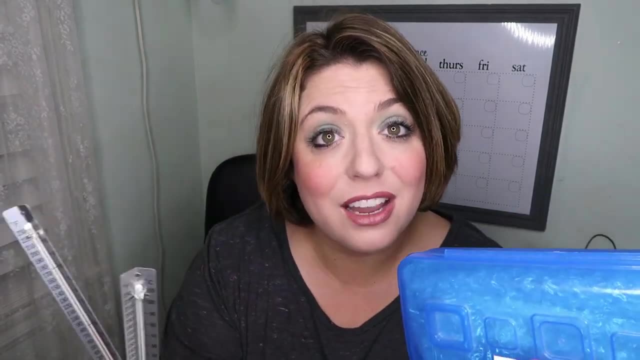 you will have a thermometer, two thermometers for each of your classes. That's all you'll need each student. You won't need one, So each of you tutors. there is nothing that you need to buy or purchase or bring to community day for the first week. I will have everything for you, All right. so in looking 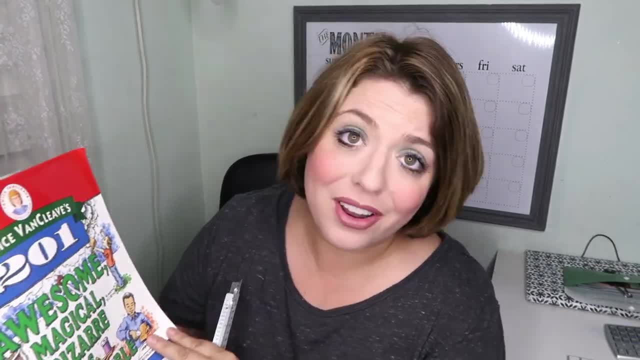 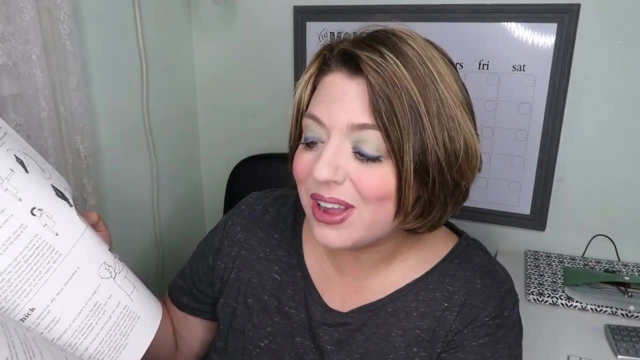 through our Janice Van Cleave 201 Awesome, Magical, Bizarre and Incredible Experiments book. we see that we are on experiment number two for week number one of CC cycle two, and it is called Shaded And the purpose of this project is to demonstrate how a planet's surface temperature 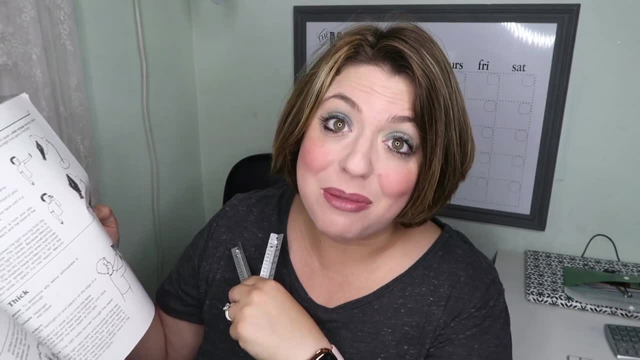 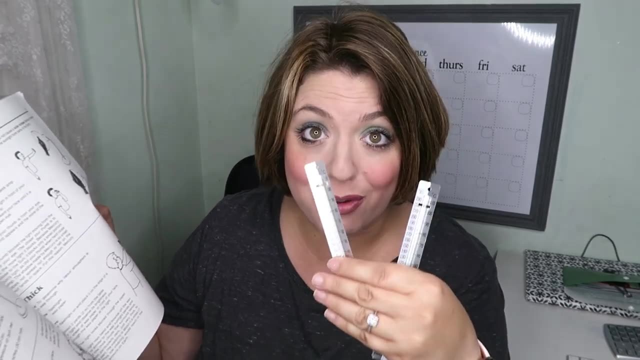 can vary. So you're going to need your two thermometers and you're going to want to come with me outside Here in just a second, But basically the procedure is that you're going to read and record the temperature on both of your thermometers after 20 minutes of being in different areas of sunshine. 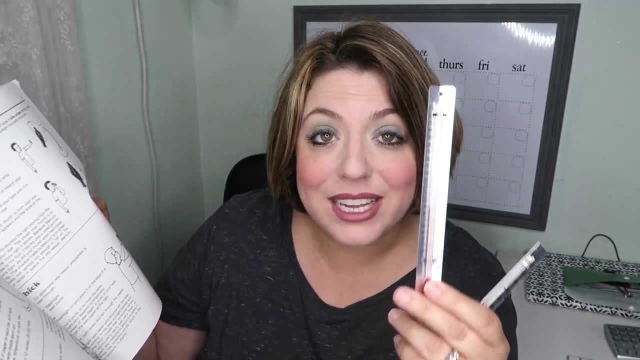 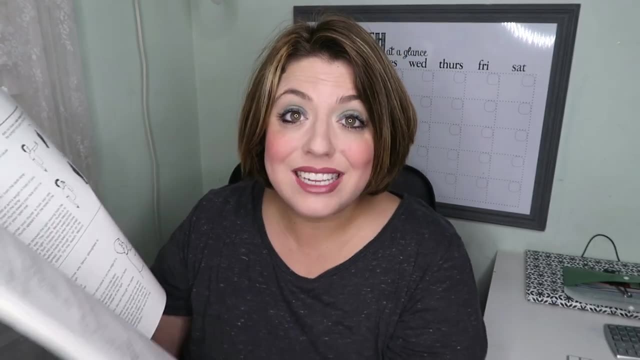 and shade. So, for example, you're going to take one thermometer and place it on the ground in the shade of a tree or another large structure, So you want the first thermometer to be placed in the shade. you're going to take your second thermometer and you're going to place the second thermometer. 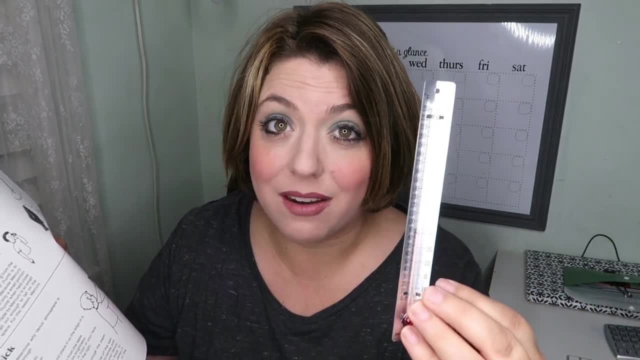 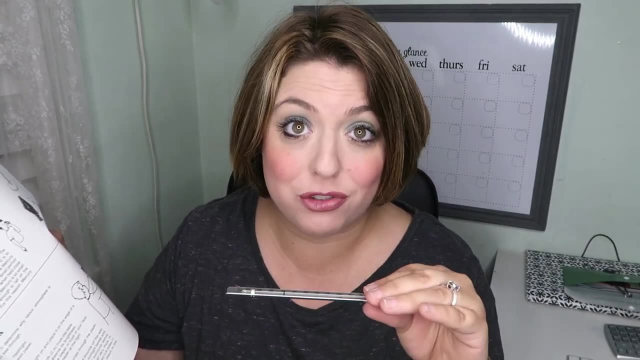 on the ground into direct sunlight, So you want it to be quite sunny and hot and warm. It is important to note, you guys, in this experiment that both the thermometers must be placed on the same type of surface, So don't put one on like a rocky surface and the other one. 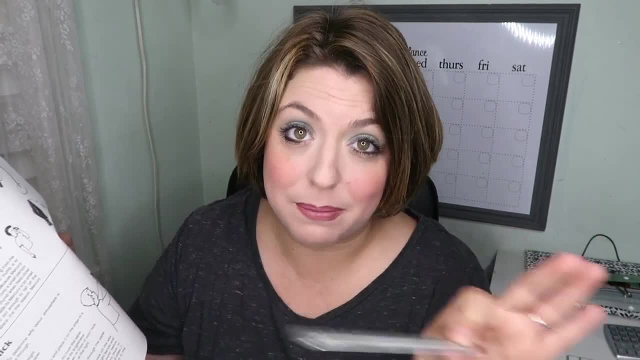 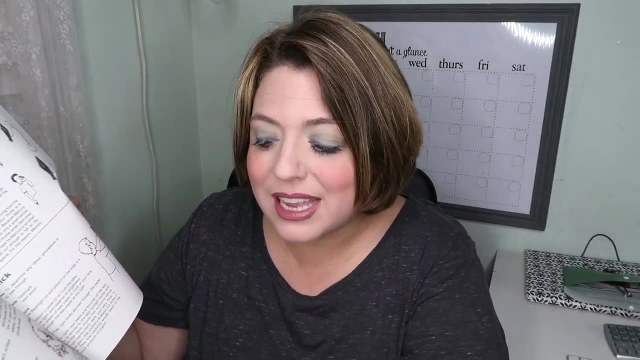 on a smooth, flat, like concrete surface. make sure they're on the same types of surface. when you do this, You're going to then, after 20 minutes, you're going to read and record the temperature on both of your thermometers And we're going to check and look at the results. 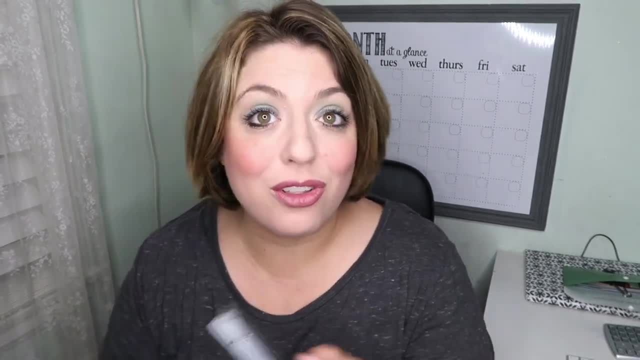 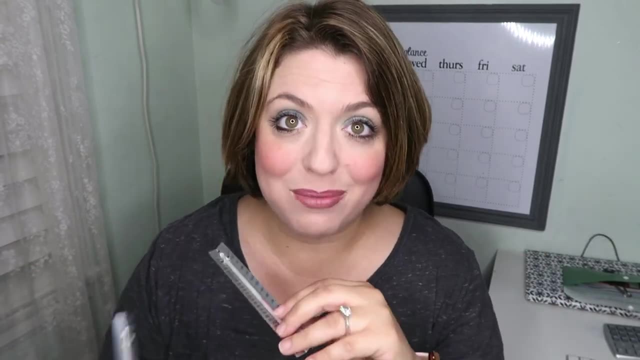 So come with me outside tutors in my community you. if you want to get here a little bit early to do this, you may do so, so you can put one in the shade and one in the sunlight, or you may have a parent do it at the beginning of class. totally up to you. let's go outside, all right you. 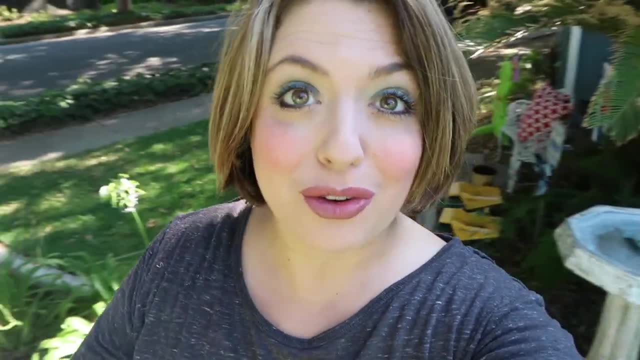 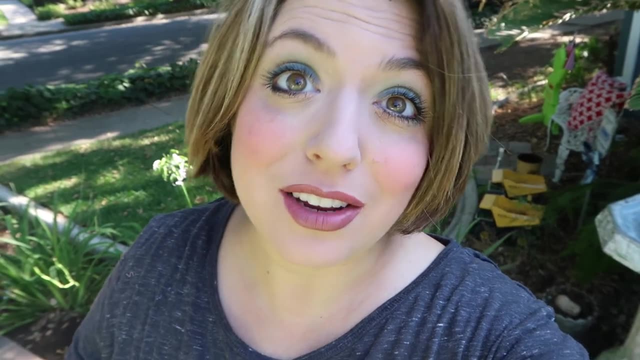 guys. so we are outside. we're actually in my front yard at my home, so this is not our community. you know area that we're meeting at that facility, but so you know we do have an area of shaded cement and sunshine cement in our community. you guys, i'm going to take our first thermometer and 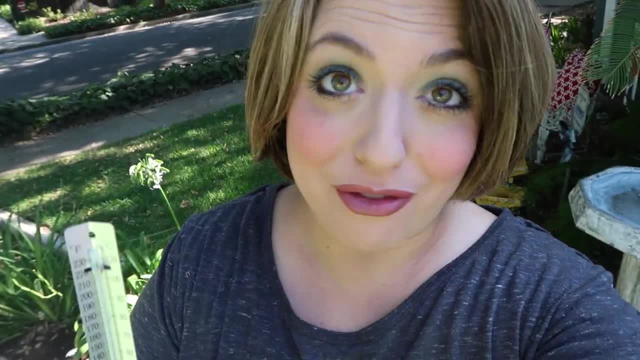 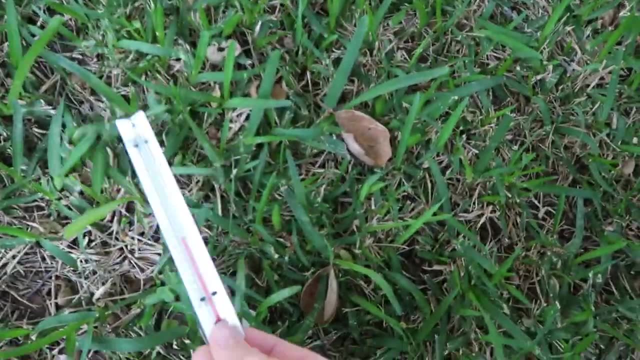 i'm going to place it on the grass, in the shaded area of the grass, because i have a lot of shade. it's early morning and we do have a lot of shade right now and sun, so here we go. so i'm in a pretty shaded area. i'm going to just place my thermometer right there in the shaded area and now we're going. 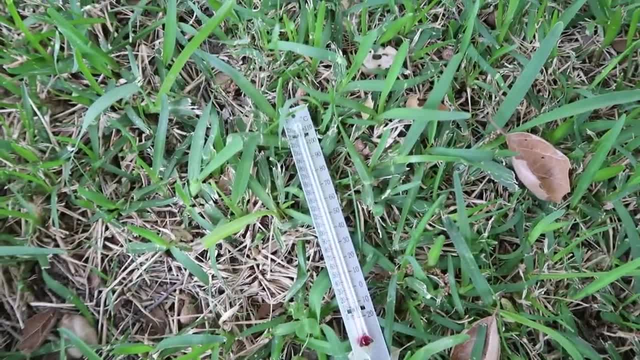 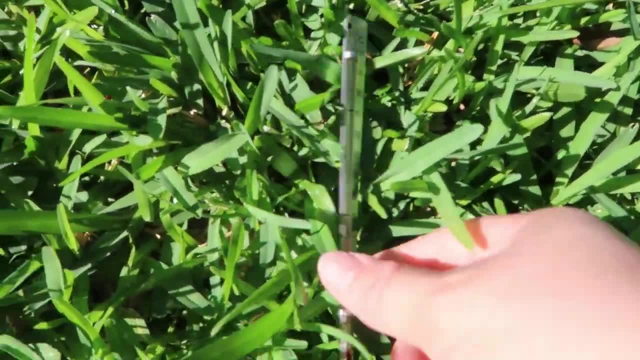 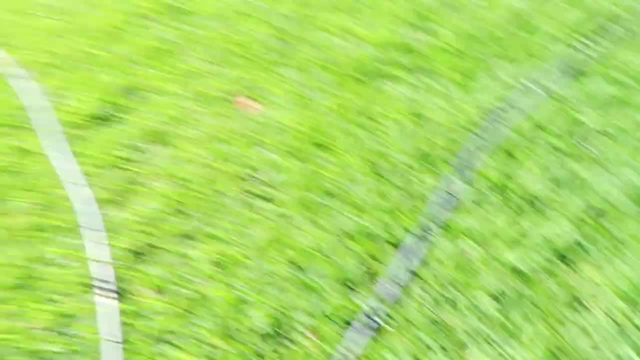 to move on to. and now we're going to move on to the sunshined area. all right, you guys. sunshiny area and thermometer number two. i'm going to place it right in the direct sunlight. there we go. my little boy is. my little boy is showing the shadow, it's okay. so here you go, here's in the sun. 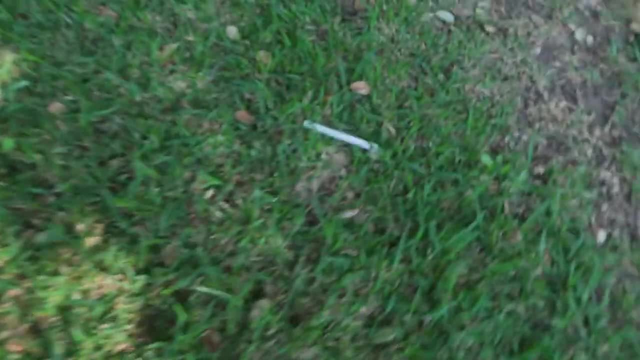 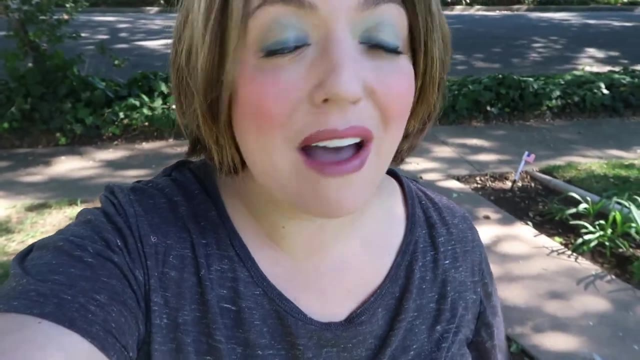 and over here we have in the shade. so so let's give it 20 minutes. i'm going to set my timer on my watch for 20 minutes and then we're going to come out and we're going to record the differences. all right, everybody, my 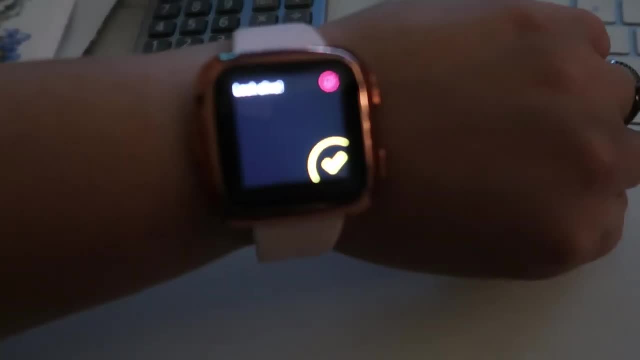 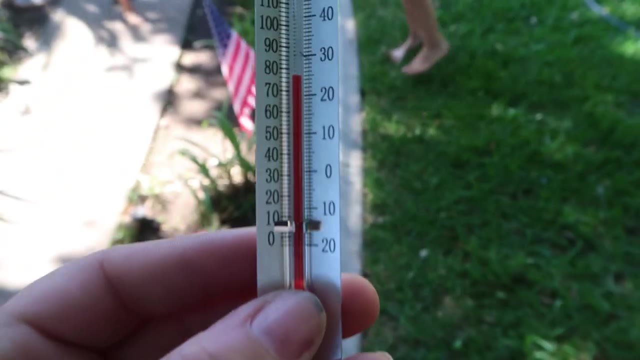 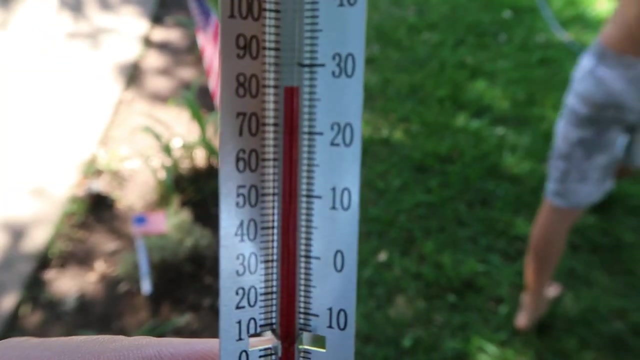 alarm is buzzing because it is 9: 34. ah, it won't focus. it is 9: 34 and it is time to check. all right, guys, we are picking up our shaded thermometer and the results are showing it is almost 80- 79. maybe that is right. on the 80: 80, we're gonna say 80, all right, 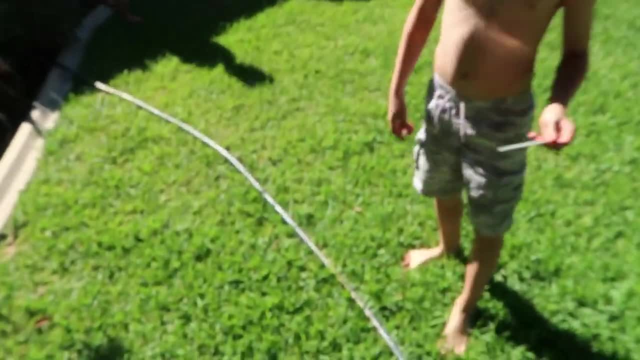 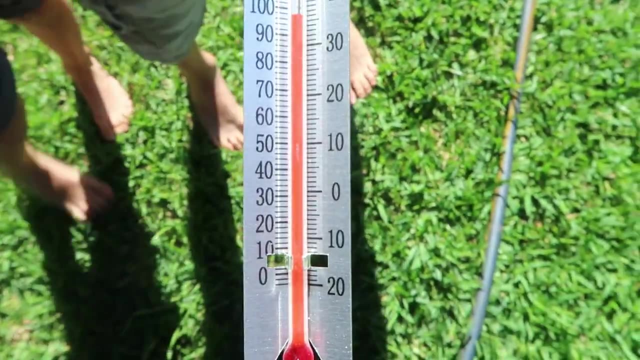 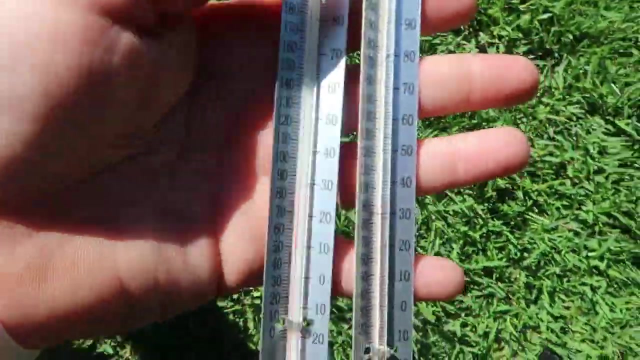 80 degrees in the shade. let's check out what the sun one says. let me see here: bud, all right in the sun, it is showing it at almost 100. do you guys see that? oh, 98. so here's the difference. okay, we have our shaded one right here, okay, and we have our sun one. let's go in and talk about the results, guys. 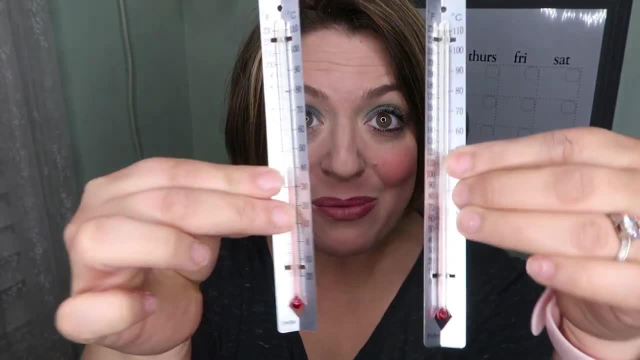 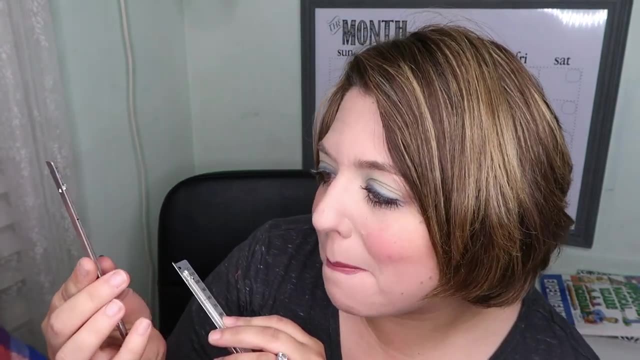 all right, you guys, we are back inside from the sunshine and here are two results. all right. so the first one was: almost this is the shaded one again. we were going to say it was about 80 degrees. i'm thinking is what we were going to say: it was almost 80 degrees. 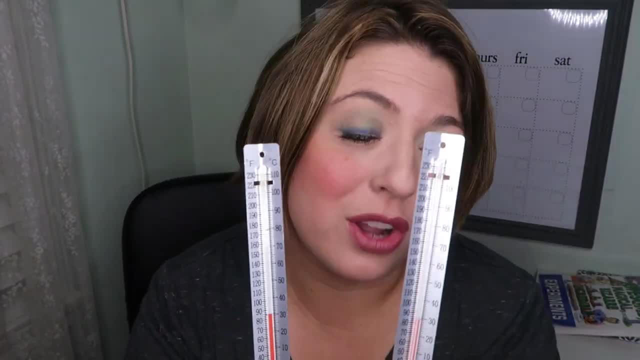 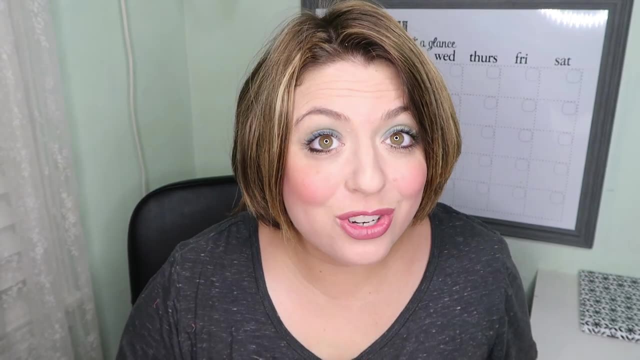 and in the sun it showed it almost 99, almost 200 degrees, which is almost 20 degrees more than in the shaded area. so that's crazy, right? so let's talk about why. so the results should show that the temperature on the surface area in the shade should be lower than the results. 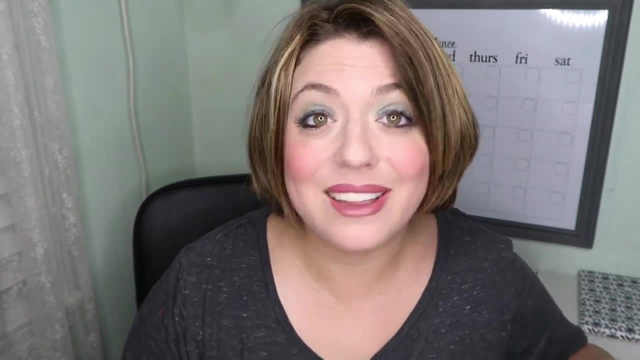 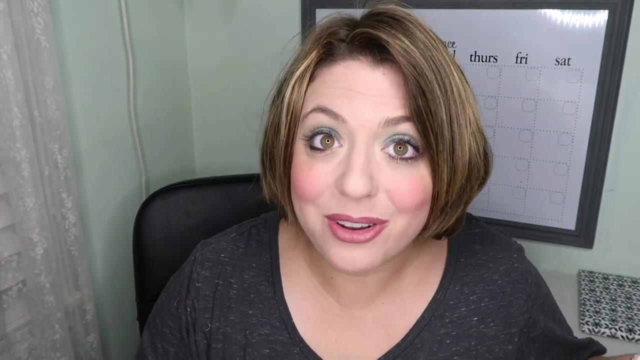 of the temperature on the surface area in the sunlight, which is exactly what we found out. so good job. okay, moving on, you might ask yourself: why is that? you have might have a student that asked that, right. well, that is, according to janice van cleve, the tree or large structure blocks some of the 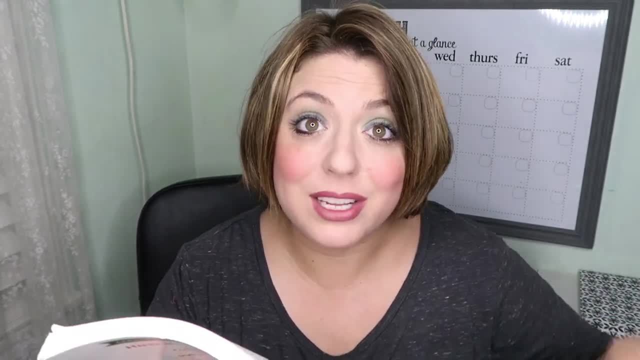 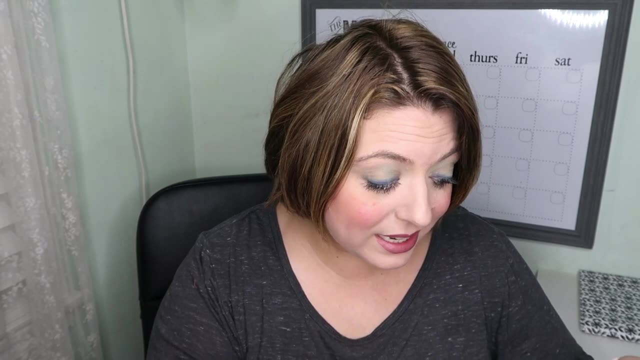 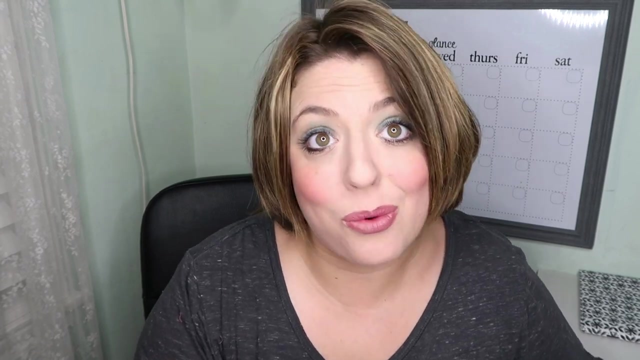 light rays. so basically, the shade under the tree blocked the light rays from the sun, producing a shaded area on the ground. this protected surface area is cooler due to the decrease in light energy received. same type of surface in direct sunlight receives more light energy and becomes hotter and 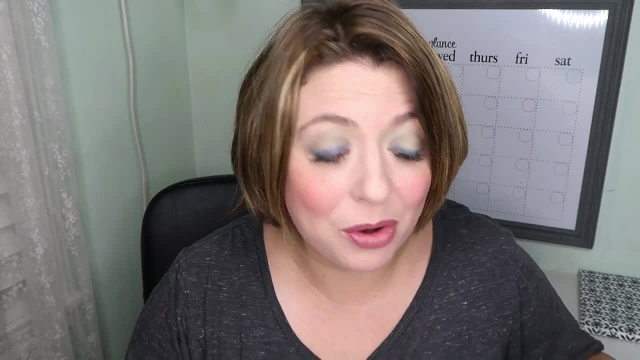 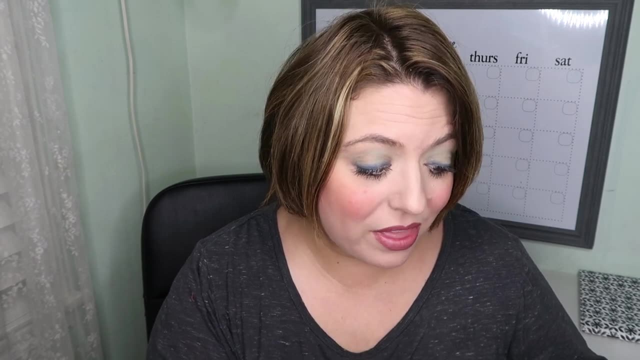 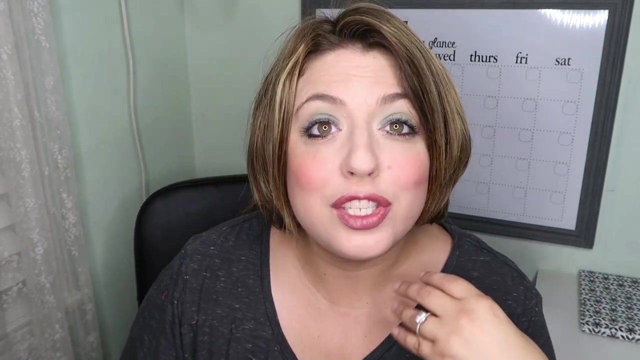 which is what we saw with the temperature thermometer. that was almost 20 degrees warmer. In the same way, the temperature of planet surfaces can vary depending on weather, the landscape and how large structures provide shade. So, for instance, we live very close to downtown LA. 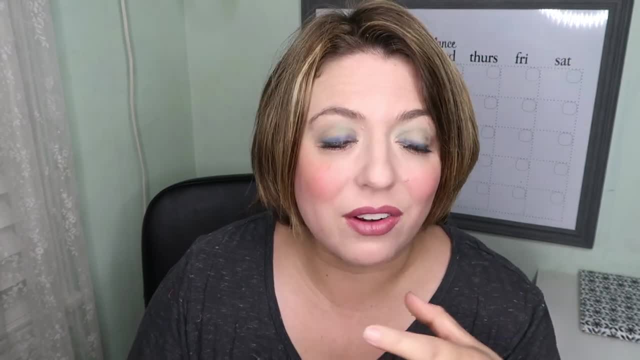 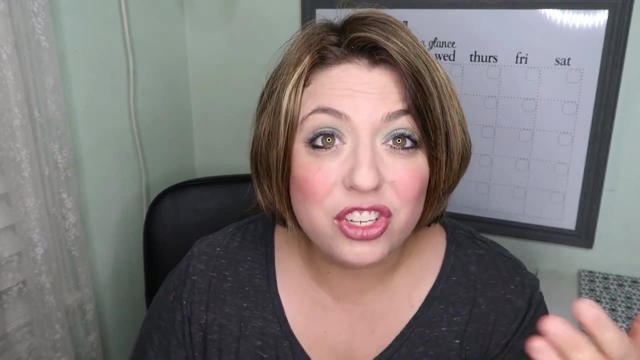 so if we are under the huge skyscrapers of downtown LA walking around, it's gonna feel and appear to be cooler and be less degrees because it's shaded by the large buildings. If we're at the beach and we're on the hot sand, 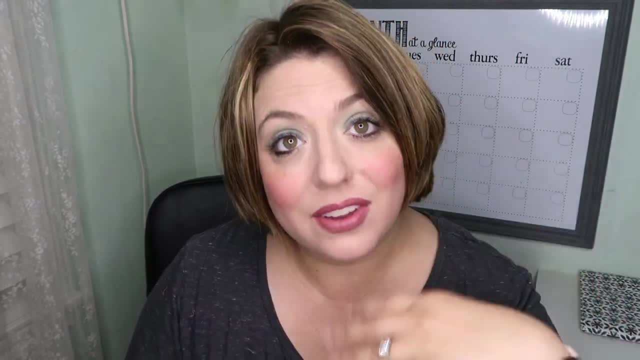 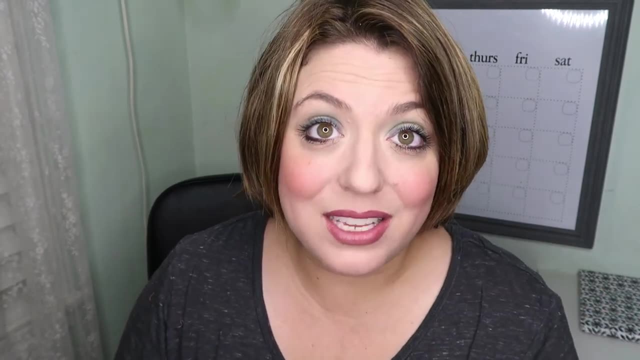 we have no shade covering us and we're directly just receiving those heat rays. So sometimes that will make it warmer when you're in front of heat or if you're laying out by the swimming pool. So I would at this point talk about with your kids. maybe some types of animals. Why do animals on a hot day? what do you see? You see your cats, your dogs are kind of over in a shaded cool area, maybe in the dirt under shade, as opposed to just laying out on the hot cement. 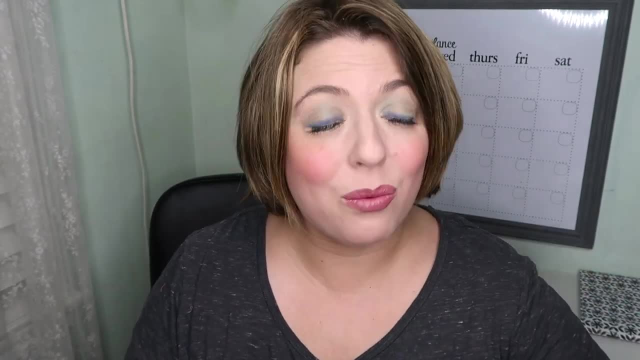 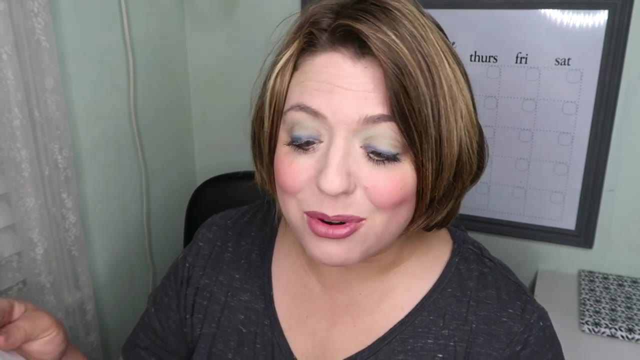 And that has to do with they want to be away from the rays of sunlight, which will make them warmer or cooler, based on if they're in a shaded environment or a sunny environment. So that is experiment number two: shaded, and let's move on to our next experiment. 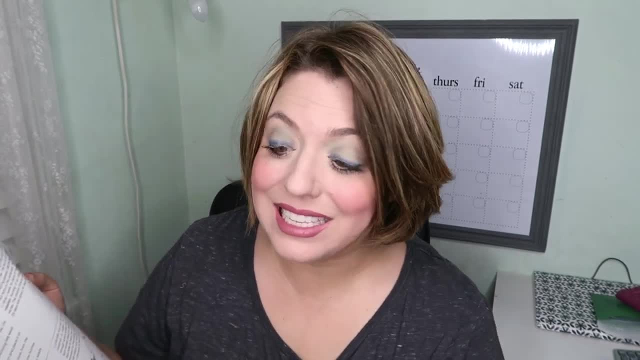 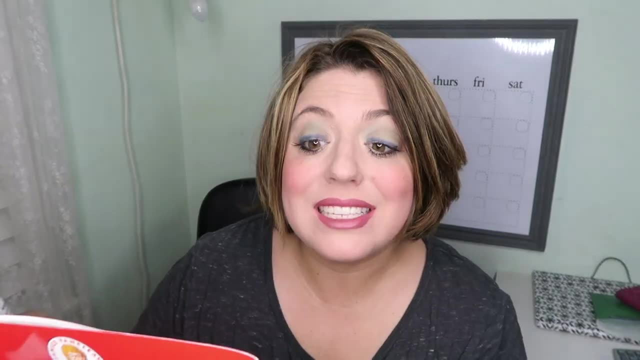 All right, you guys. so the second experiment for week two in CC cycle two, you will be doing a. it's number 17 in Van Cleve and it is called Same Place. The purpose of this is to determine why satellites. 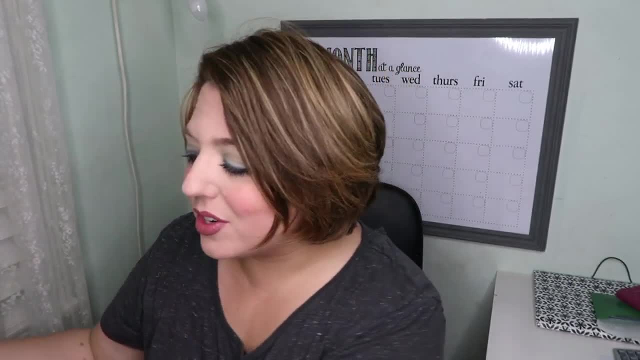 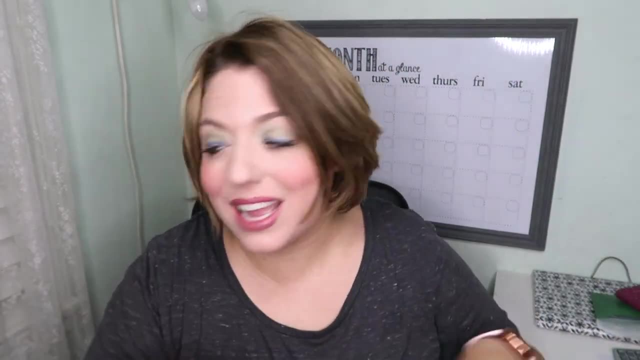 appear to be stationary and in one place. So what you're gonna need, your materials for this- are going to be a rope or a string or yarn- Look at my cat going at this, you guys- But basically you're going to want to have. 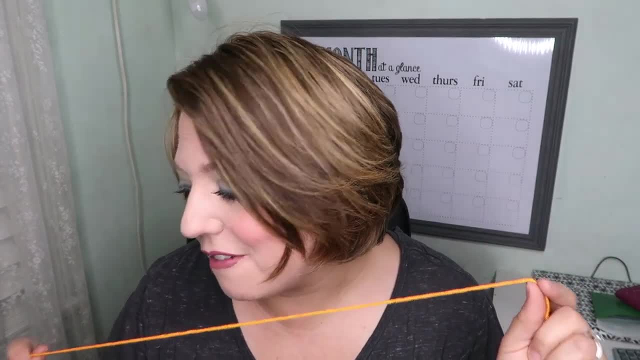 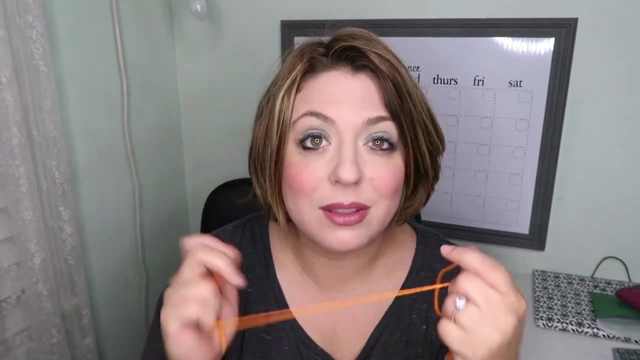 about three yards or three meters long of some sort of- I was gonna say- yardage, some sort of yarn or rope or some twine or something thick and nice like that. And so for this one, I'm actually not gonna take my kids outside to do this, because I don't know. 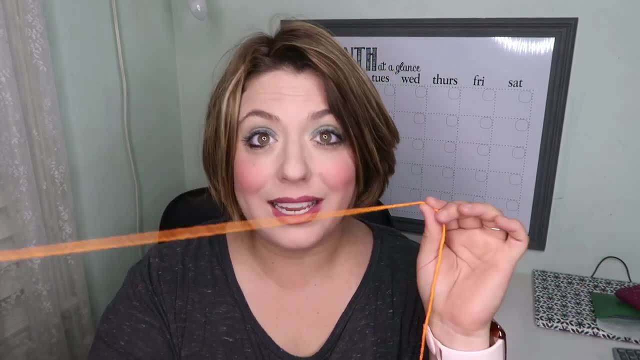 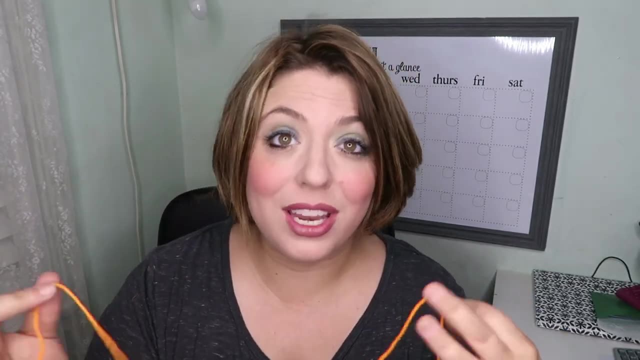 that we have enough tree space here at our home, but I'm gonna describe it to you in detail and in depth. Basically, you're gonna go out in an open area outside, So find something in our community or in your community that looks just like this: 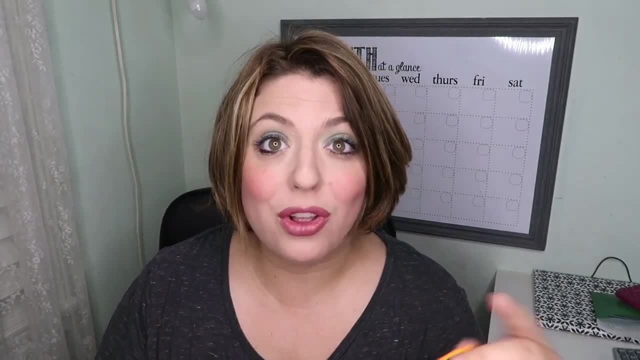 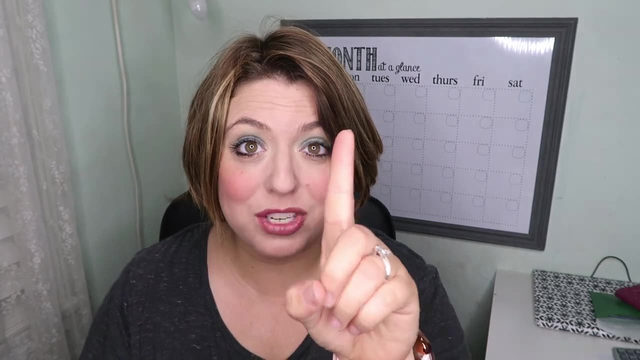 You're going to want to use a tree or a light pole or a light post or some other object that's stationary and standing up and down, And you're going to want that to represent the earth. okay, So if this were my tree or my stationary object, 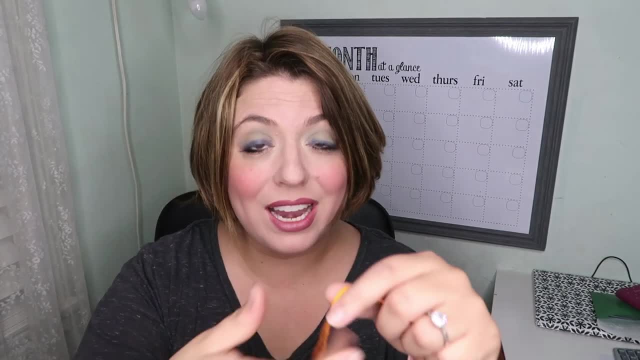 this would be the earth, okay. So you're gonna want a helper to hold onto one end of the rope as you hold onto the other end of the rope. So you'll need one child to help you out with this and maybe you can take turns. 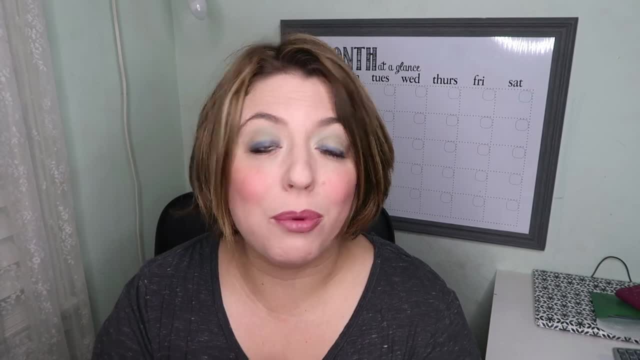 We're gonna do this in our community today and have each kid kind of try it with a parent or with a helper, once you've demonstrated first. So you'll need your helper to hold on one end, You'll need to hold onto the other. 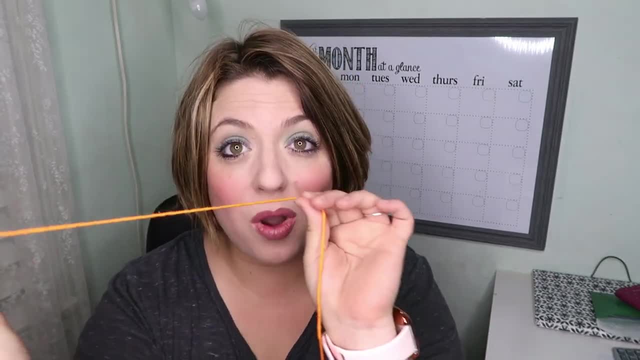 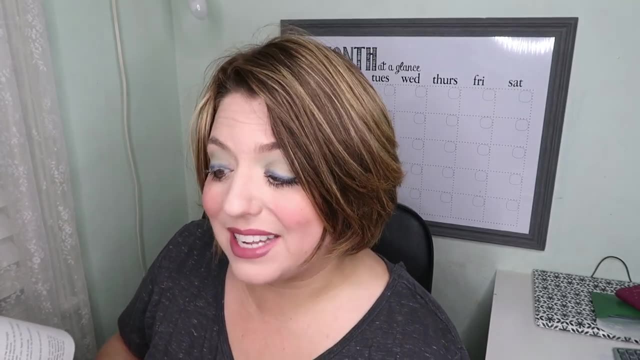 So you're gonna want to have your helper stand near the tree and you're going to want to walk at a pace around the tree, holding the rope and maintaining it tight. I'm gonna read this part: You're going to want to walk at a pace. 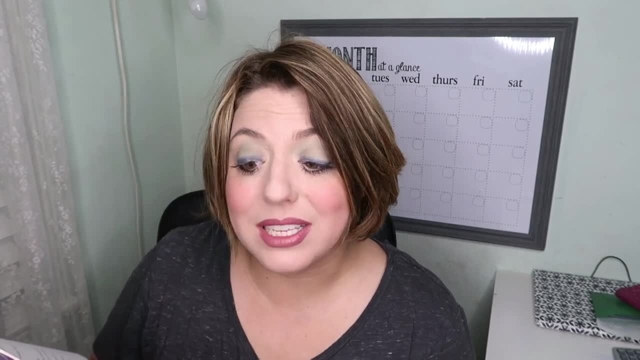 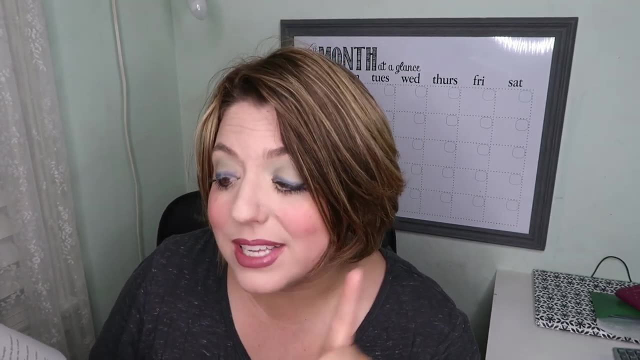 that keeps the rope tight and in a position so that you are in line with the same point on the tree as your helper. The whole time you're going around, you're gonna want to be doing this. The results of this: the person in the outside. 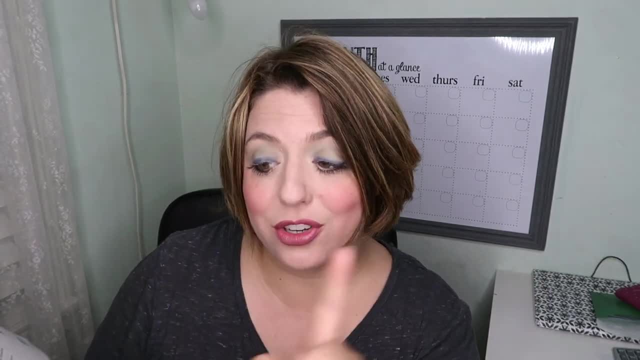 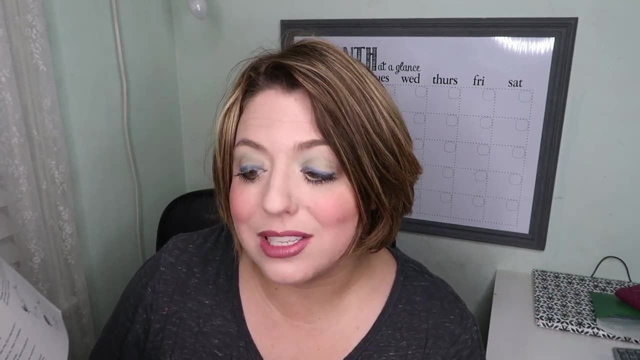 circle, the one moving. okay. the one moves faster but stays in line with the person moving in the smaller inside circle. Why is that? The distance around the outside of the circle is larger than the circle near the tree. A faster speed is required to travel around. 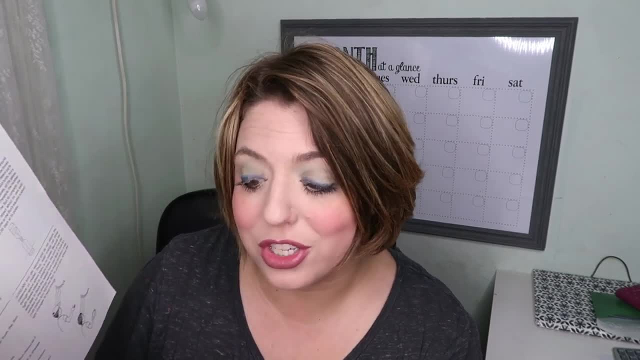 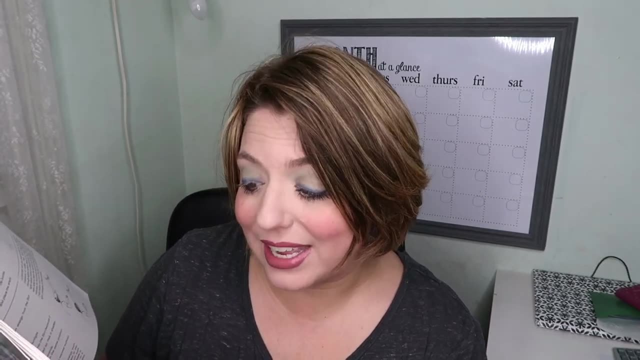 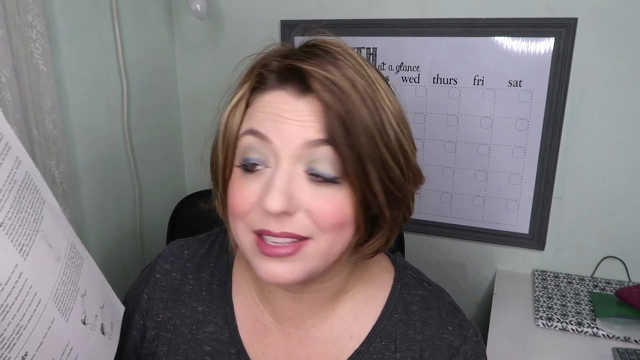 the larger circle in the same time that the person closer to the tree travels around the smaller circle. This is known as Geostationary Operational Environmental Satellites, or GOES, and they are placed at about 22,500 miles above the Earth and they move at a very fast speed.